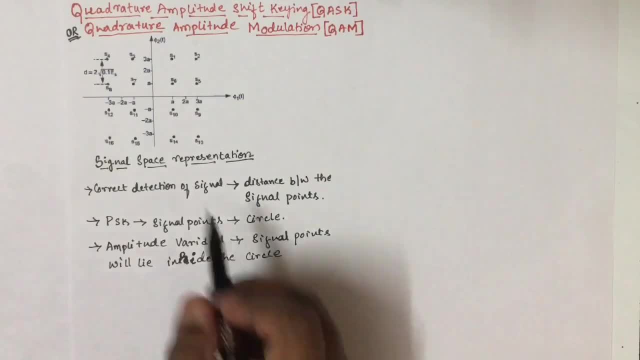 If amplitude is varied, at that case the signaling point will lie inside the circle of the signal space. If the signal points lies inside the circle, at that case it will increase the noise immunity of the system. So if the signaling points lies inside the circle, at that case. 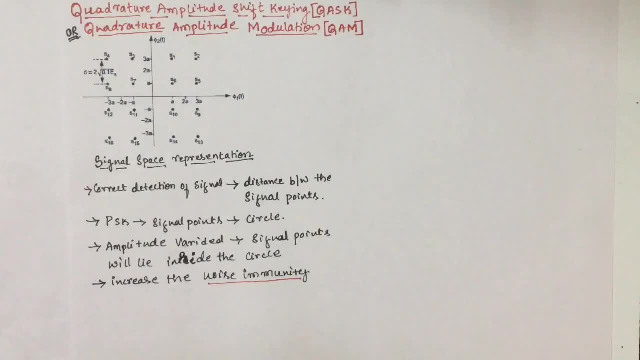 the noise immunity of the system will be increased. So if the signaling points lie inside the circle, at that case it will increase the noise immunity of the system. This type of system are known as QASK or QAM. Now let us understand the geometrical representation of QASK or QAM signal. 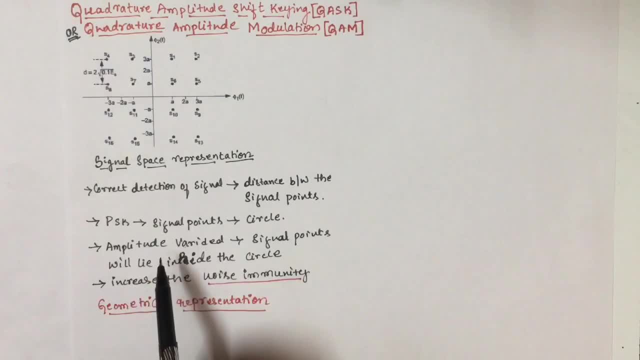 Figure shows the geometrical representation of QASK signal. Let us consider 4-bit symbol, then there will be 2 to the power of 4, which will be equal to 16 possible symbols If we consider 4-bits. for example, let us consider the bits 1011010.. 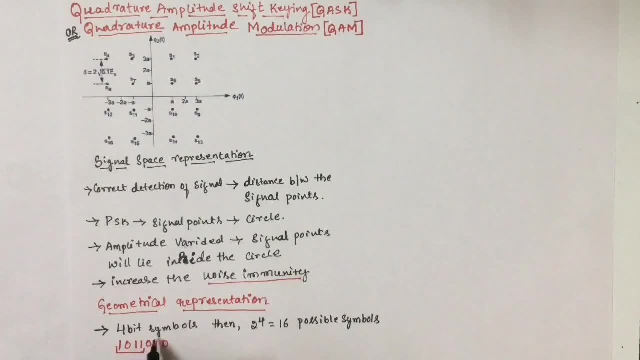 In this: if we consider 4-bit as 1 symbol, then 2 to the power of 4 will be having 16 possible symbols In QASK. these 16 possible symbols are represented in signal space as shown in this figure. 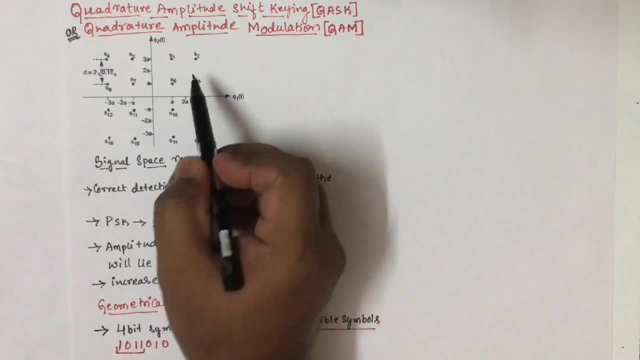 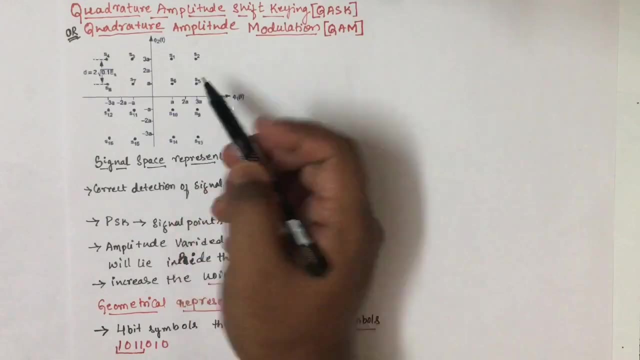 As you can see here, these 16 possible symbols are represented in signal space. As you can see here, these 16 possible symbols are represented in signal space, as shown in this figure, in four quadrants, and each quadrant is consisting of four signal points. 16 possible symbols are: 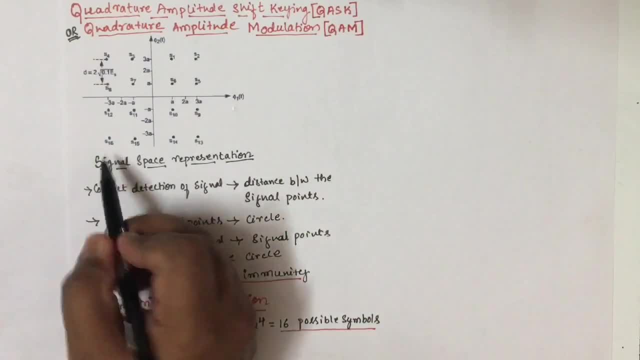 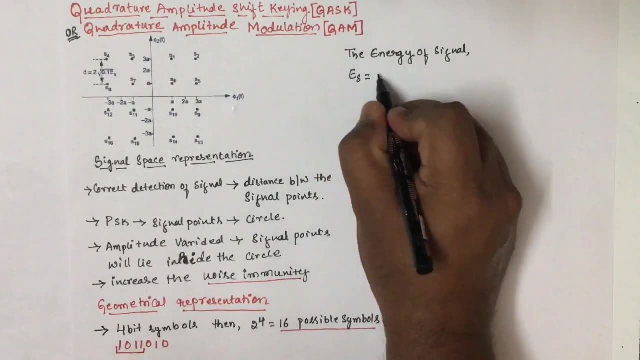 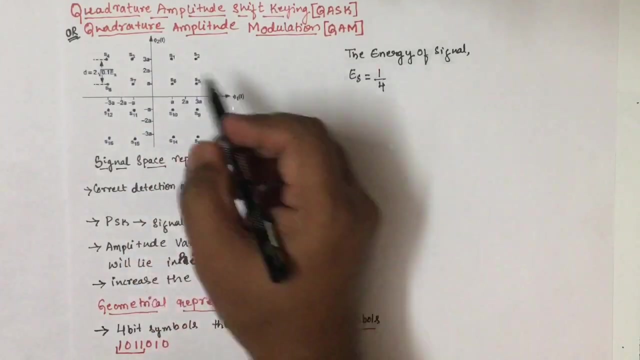 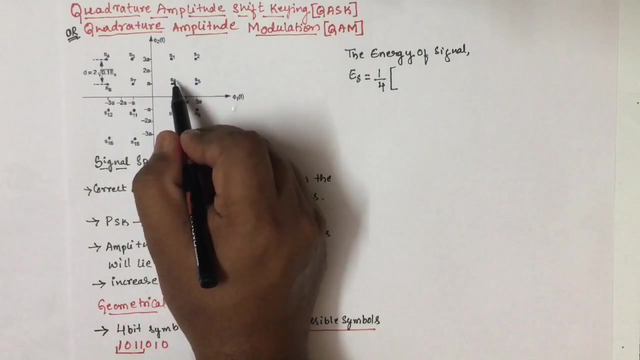 represented as S1 up to S16.. The energy of the signal can be given as ES. that can be written as 1 by 4 because in each quadrant there are four signal points. To take the average of the energy, we are writing it as 1 by 4 into. for each signaling point we will take it as x square. 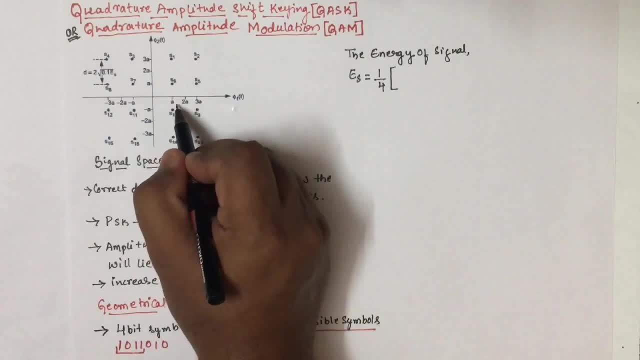 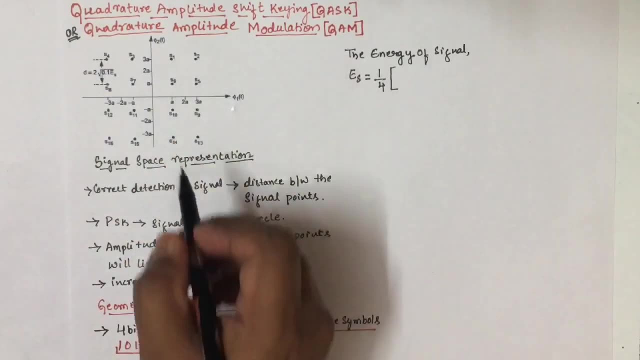 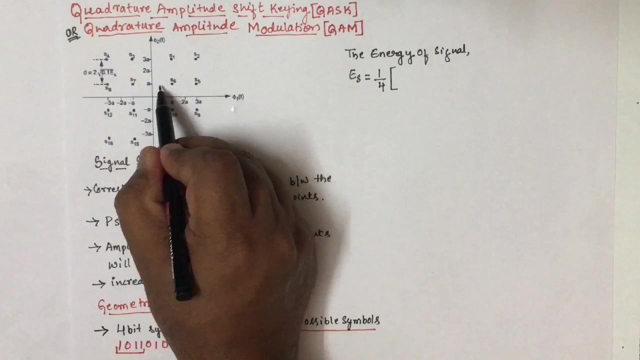 and y square, which means we will take the value in x and we will take the value in y and we will square that value and add those values. So, for example, if we consider S6, the value of the signaling point in x axis is a and the value of the signaling point in y axis is a. So we will. 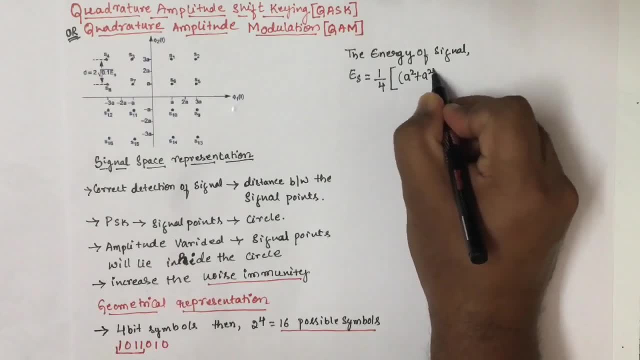 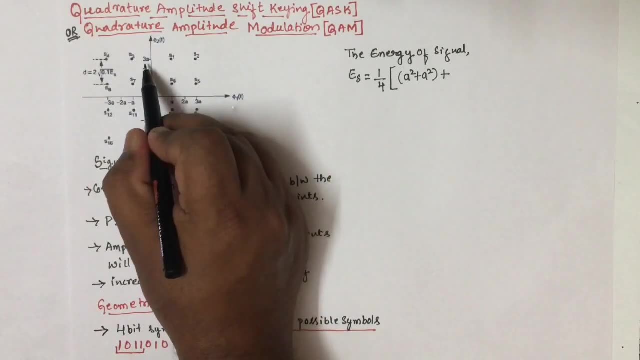 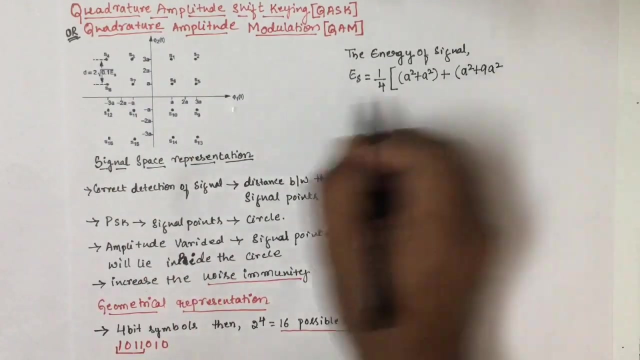 take that as a square plus. a square plus. we will consider S1. the value in x axis is a. the value in y axis is 3a, So we can write that as a square plus 9a square, because we are squaring this value. 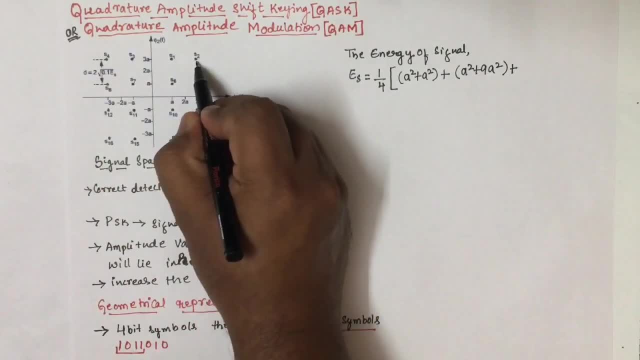 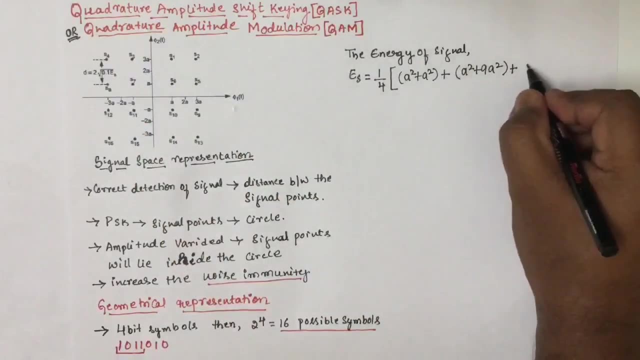 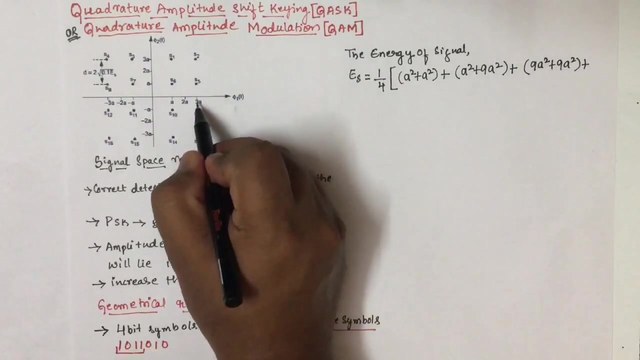 plus. for signaling point S2, we will take it as 3a in x axis, 3a in y axis, So we can write that as 9a square plus 9a square plus. for S5, we will take 3a in x axis and a in y axis. We will write that: 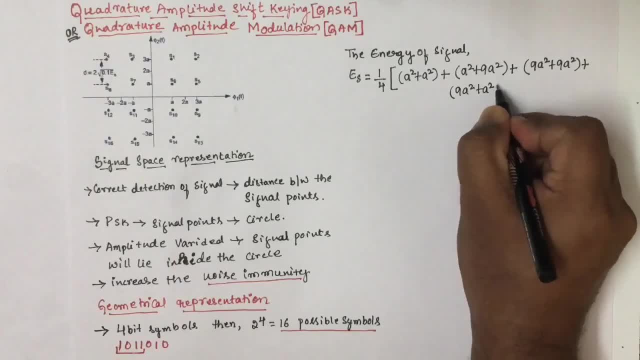 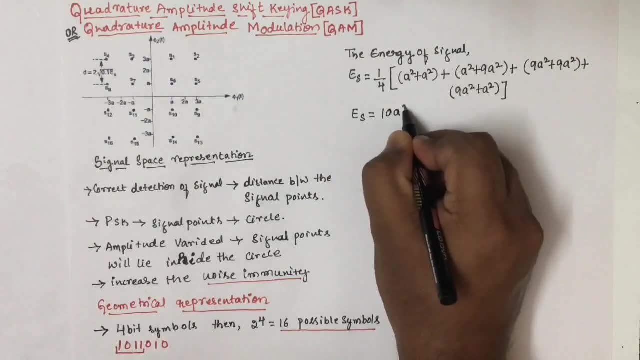 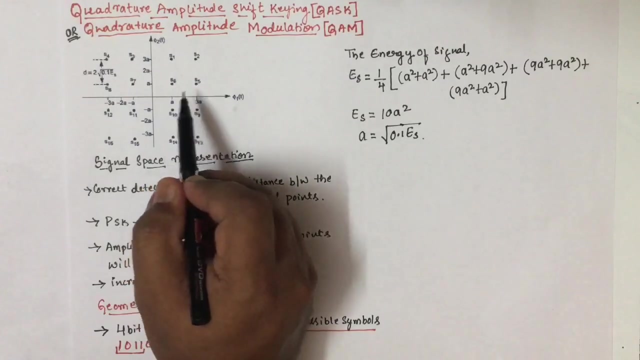 as 9a square plus a square. If we simplify this value we will get: ES is equal to 10a square. From this we can find a is equal to square root of 0.1 ES. If we observe this representation here, the distance between the neighboring points is 2a. 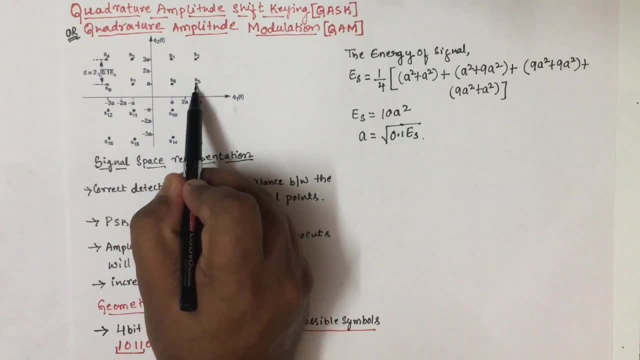 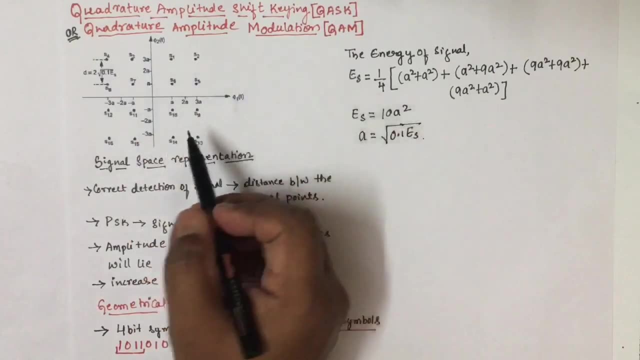 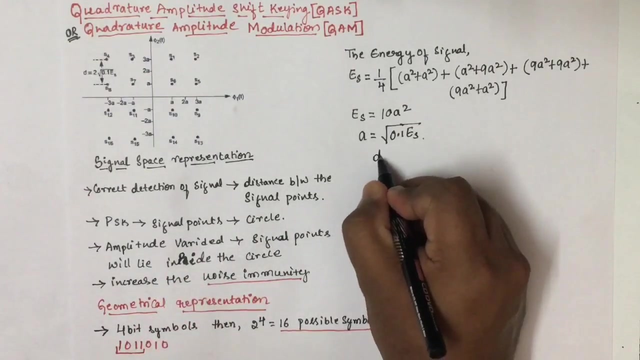 So if you consider this signal point and this signal point, the distance is 2a. Similarly, the distance between these two signal points are 2a. So likewise for all the signal points, the distance is 2a. So we can write: the distance between the signal points are 2a, So the distance between each. 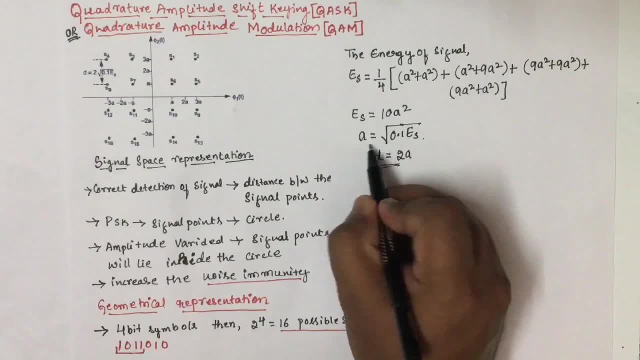 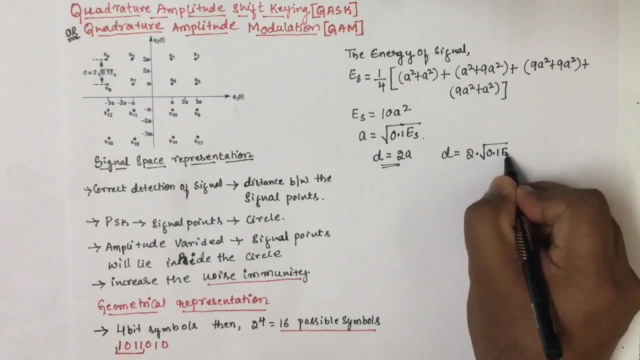 signal point is 2a. We have calculated the value of a, so we can write: D is equal to 2 into square root of 0.1 ES. so we can write this as: D is equal to square root of 0.4 ES. This is the same value. 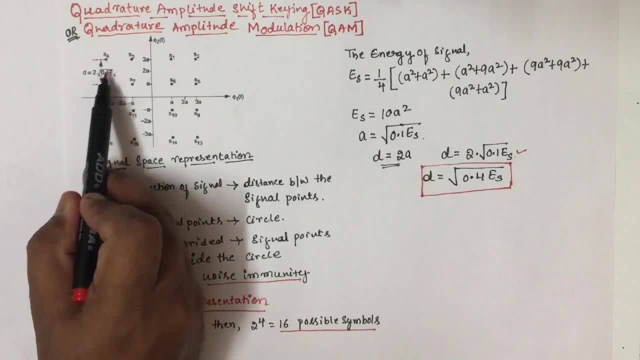 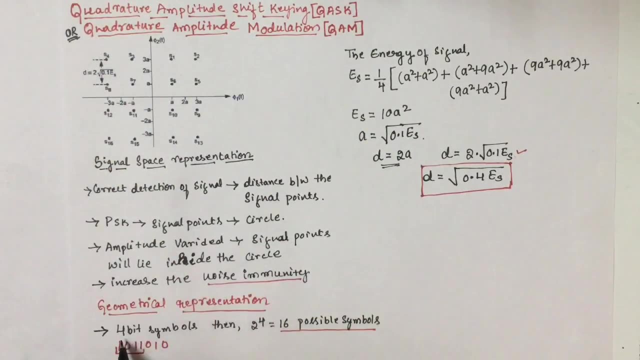 which is written in this representation, D is equal to 2 into square root of 0.1 ES. So this is the distance between each signaling space. We know that there are 4 bits in each symbol. Therefore we can represent symbol.